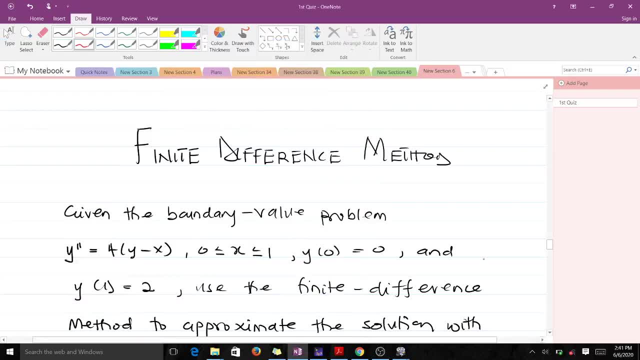 Hello and welcome to today's lesson. So in today's lesson we are going to talk about the finite difference methods used in the solving of ordinary differential equations with boundary value problems, boundary value conditions in numerical analysis. We are going to take a question to explain this concept. So the question reads: given the boundary value problem, y prime prime equals 4 times y minus x, with x lying between 0 to 1 and y of 0 equals 0 and y of 1 equals 2, we have to use a finite difference method to approximate the solution with h equals 1 over 4.. 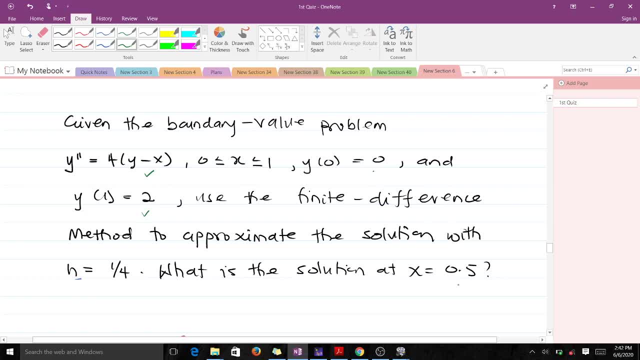 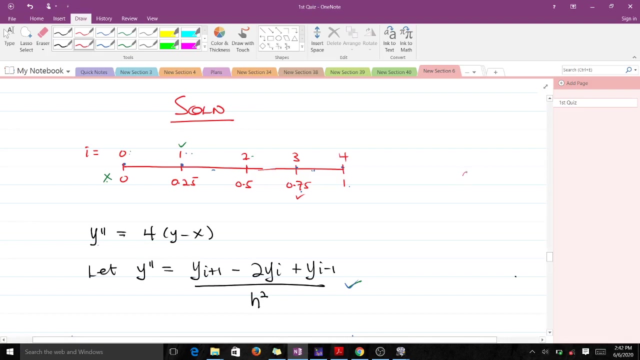 And after that we have to find the solution at x equals 0.5.. I hope you get it. So let's note: we have this interval here, We have these boundary conditions here And this is our differential equation. So, solution: recall that our interval was between 0 to 1.. We had x lying between 0 to 1.. So that's 0 to 1.. And we had our h to be 1 over 4.. 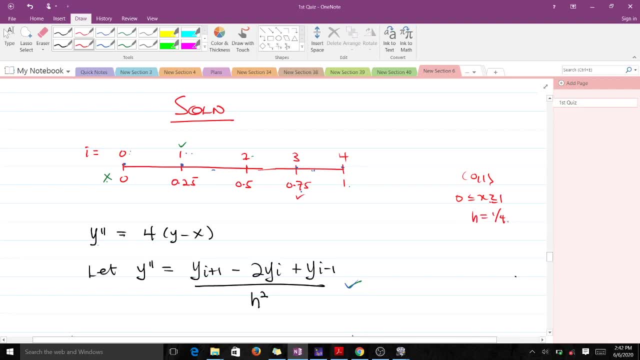 Our h being 1 over 4 means that our interval has been divided into 4 equal parts. So dividing the interval 0, 1 into 4 equal parts is going to give us 0,, 0.25,, 0.5, and 0.75 up to the 1.. 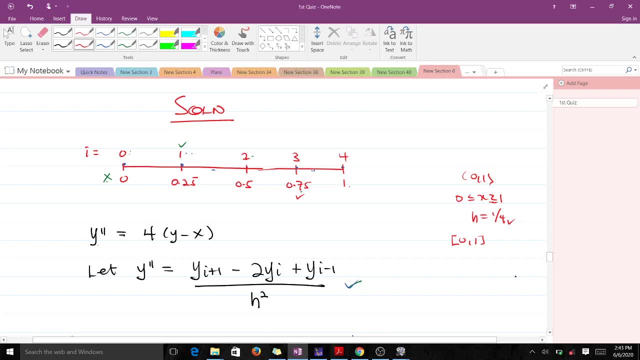 So from here to here we add our h, So 0.25 plus 1 over 4 gives us 0.5.. And we do that. We have 5 nodes here. So this node, this, another node, We have another node here, another one here and this. 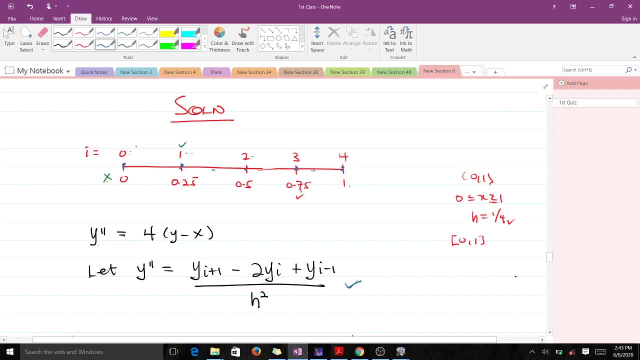 So we decide to name these nodes. So we name here 0,, 1,, 2,, 3, and 4.. So after that we know that this was the equation which was given to us in the question. So what we do is that we try to approximate the second derivative here with the essential difference formula. 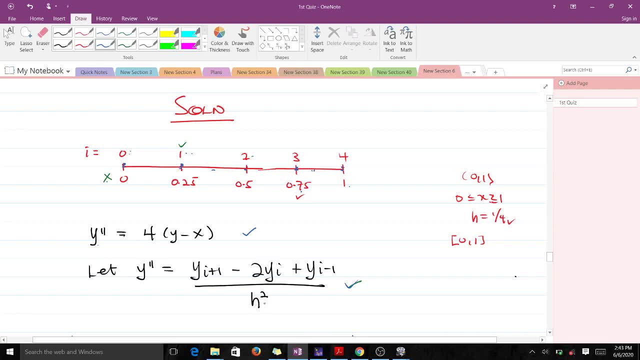 That's y i plus 1 minus 2, y i plus y i, y i minus 1 over h squared. We know that h has been given to us in the question, So with this approximation now let us try to put it inside our main equation. 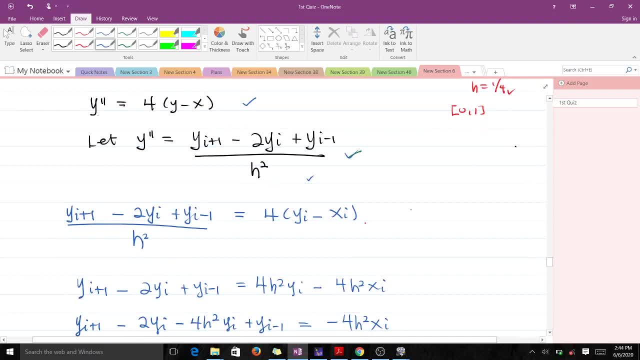 It is going to give us y i plus 1 minus 2, y i plus y i minus 1 over h squared. So whatever you find here, you put this here And this will be equal to 4 times y i minus x i. 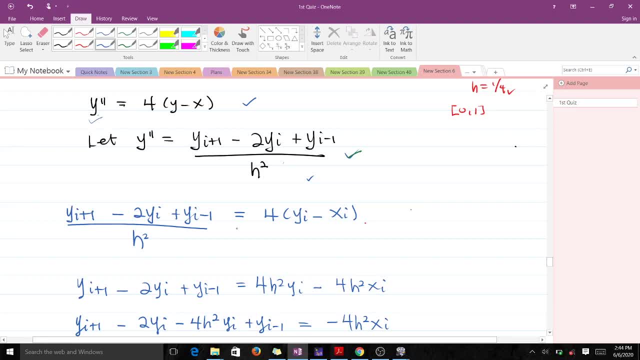 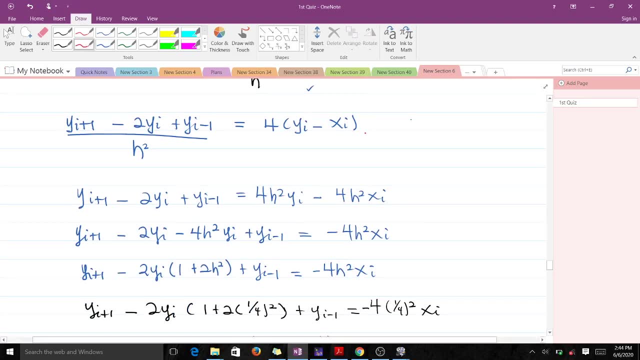 I hope you get it. So when we get it then we can decide to: you know, do some odd Algebra here. So we multiply 2 by h squared And that gives us this result. Then we try to bring y, i here. 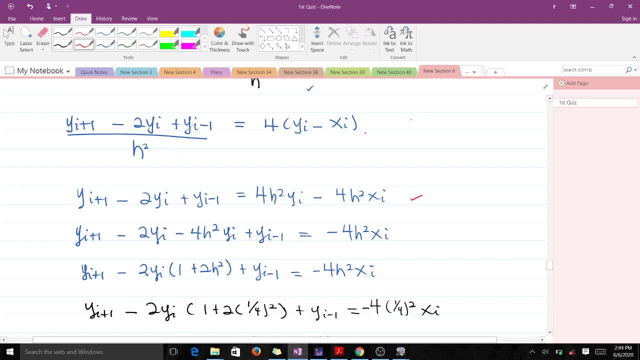 And this gives us this, And we try to bring this to the left-hand side And after that we try to, you know, factorize 2 y i from here. So doing that, we get something like this And we know h was given in the question to be 1 over 4.. 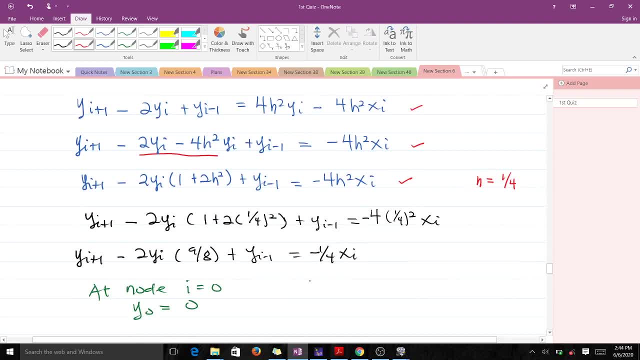 So putting in the 1 over 4 inside wherever we find h gives us this, which can finally be simplified into this, But I mean this happens to be the finite difference equation for this particular question. We had five different rules, So with i equal 0,, 1,, 2,, 3,, 4, and 5.. 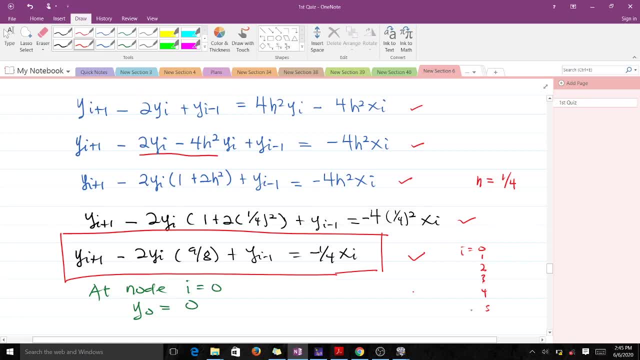 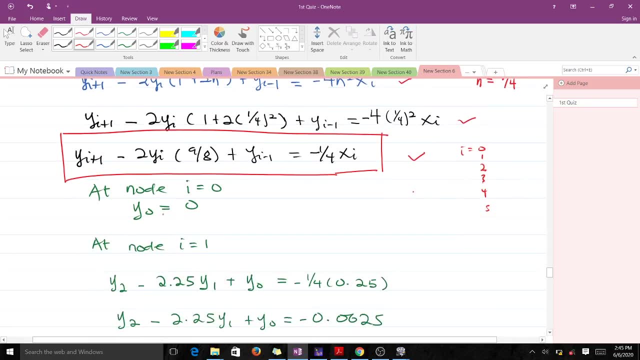 So we are supposed to find equations for, or find a difference equation at all these nodes. So at the node i equals 0, it is going to give us y not equals 0. That is the starting initial boundary condition which was given to us. 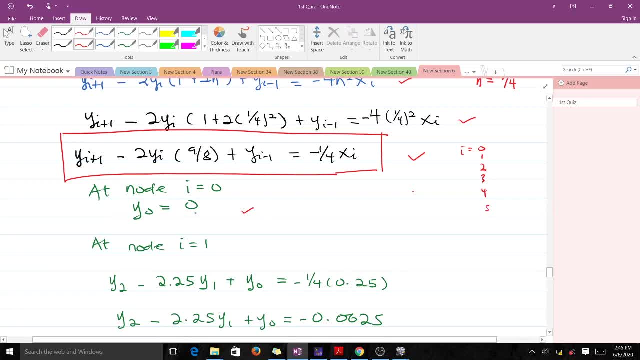 So there is it. So at i equals 0, y not equals 0.. Recall that the boundary conditions were y of 0 equals 0 and y of 1 equals 2.. So, at the node, i equals 0, it is going to be this: 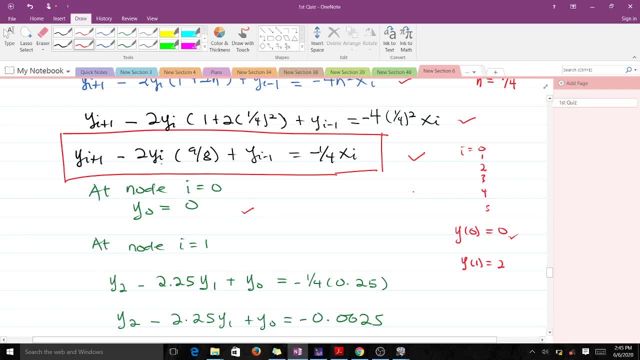 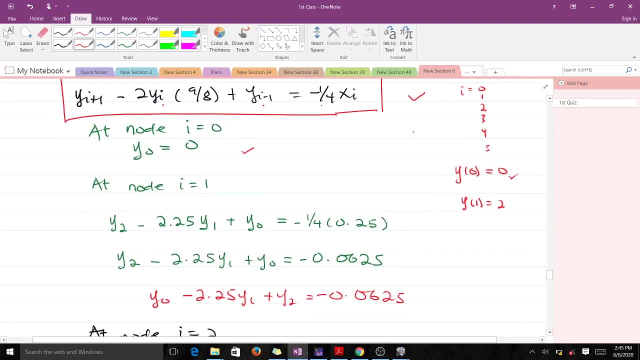 Then at the node i equals 1, we will put 1 wherever we find. i here That is going to reduce our equation to y2 minus 2.25. y1 plus y0 equals negative 1 over 4, 0.25. 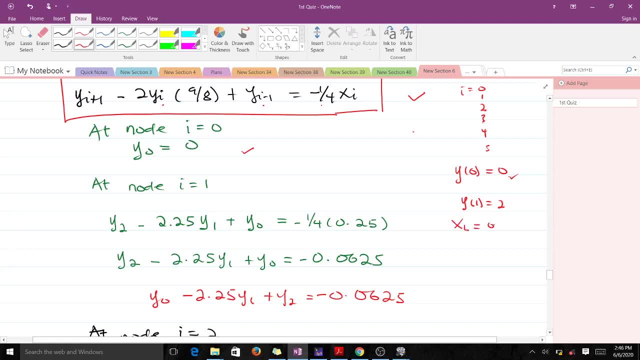 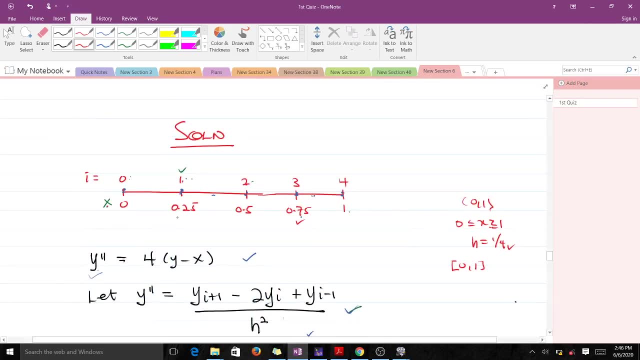 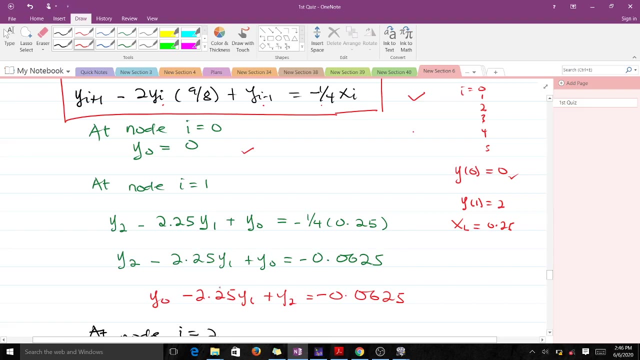 0.25, because x1 is equal to 0.25.. Let's see why. So you see, x at i equals 1 is 0.25.. So we put that inside our equation and when we do our algebra we end up with this particular equation here. 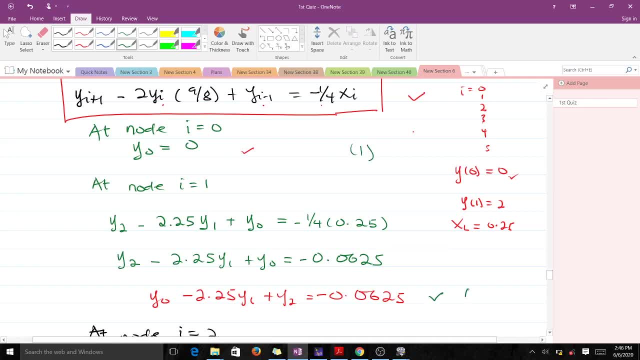 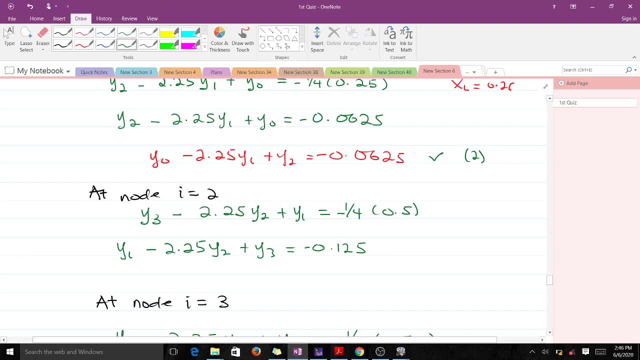 And this becomes equation 2.. Recall: we have equation 1 here. This becomes equation 2.. Then we go to the node at i equals 2.. We make substitution. We get y3 minus 2.25, y2 plus y1, which will be equal to negative 1 over 4 x2.. 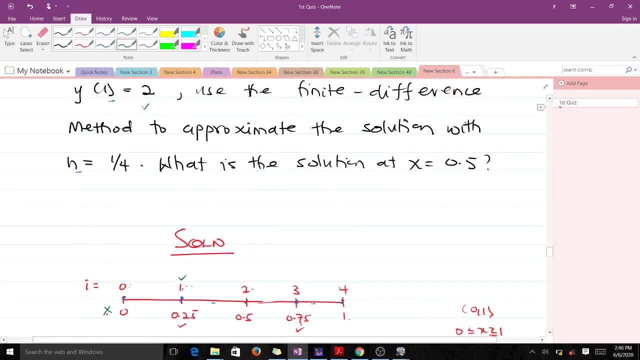 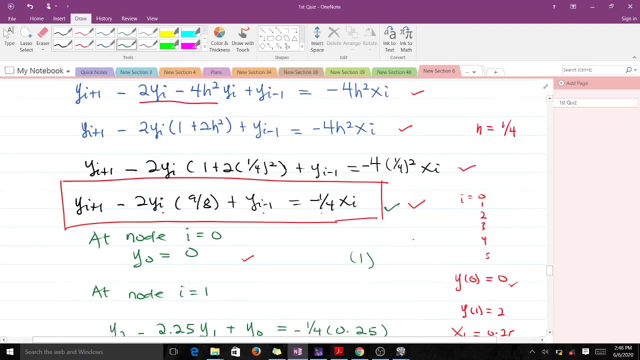 x2 is 0.5, so we can check it out from this place: x2 is 0.5. And note that all our i's we are putting it inside this equation because this is our difference equation for the question. 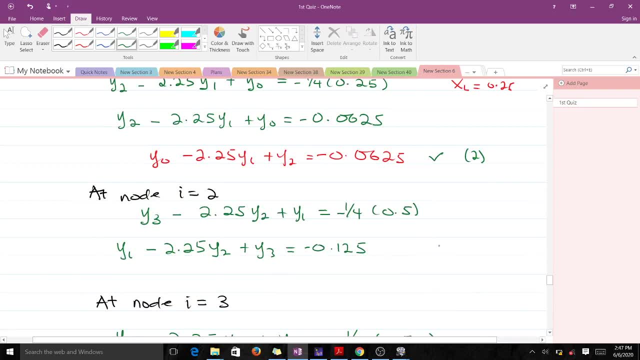 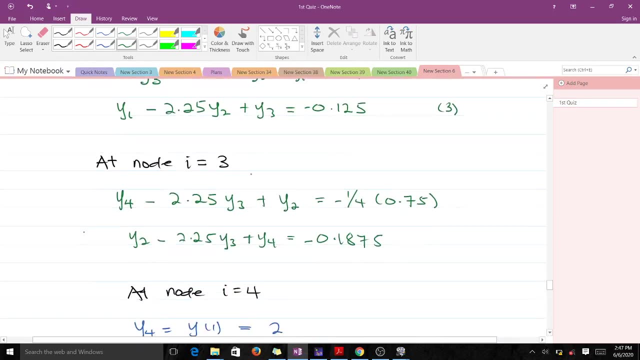 So that is going to give us this equation here, which is going to be equation 3.. Then, at node i equals 3, we make our substitution again and we get this here, which happens to be equation 4.. Then, at the node i equals 4, we are going to get this one. 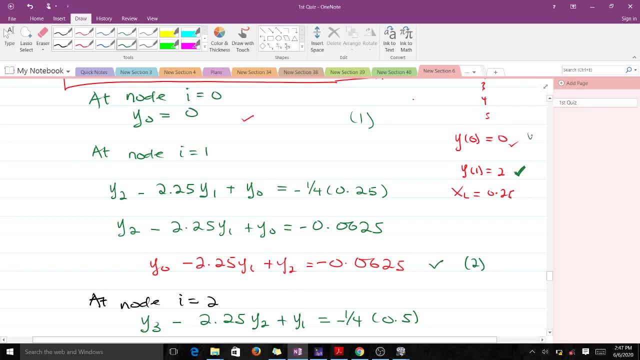 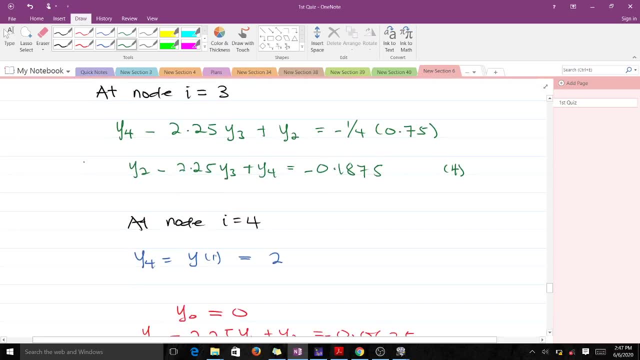 Because we had two boundary value conditions. So this is for y naught and this is for y4.. So at the node i equals 4, we are going to get y4, which is equal to y of 1 will be equal to 2.. 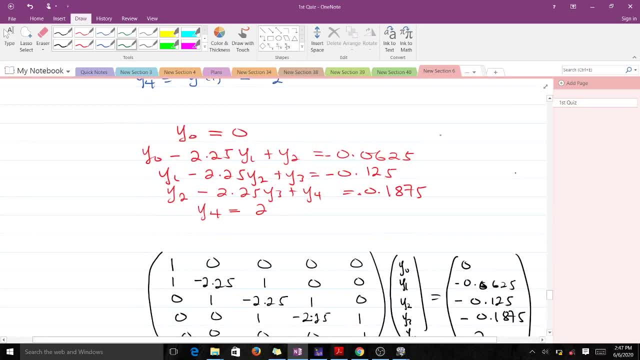 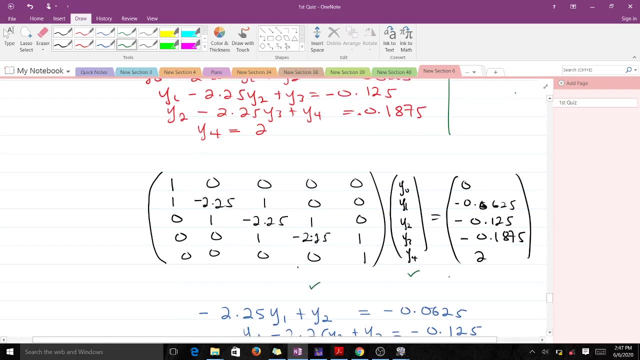 So that means that after doing this, we have five equations And these are our five equations. So we are supposed to solve for this for y naught, y1, y2, y3, and y4.. So putting this inside the matrix form gives us this, as we can see here. 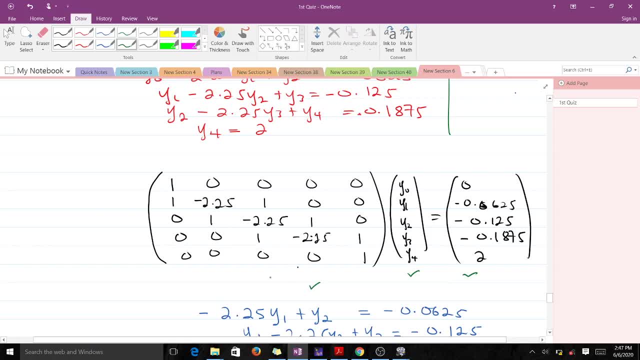 And we can see that with the coefficient matrix that we have here- let's name it a- We can see that it is tridiagonal. it is tridiagonal, right? So that means that finding for y naught y1, y2,, y3, y4, we can use the Thomas algorithm. 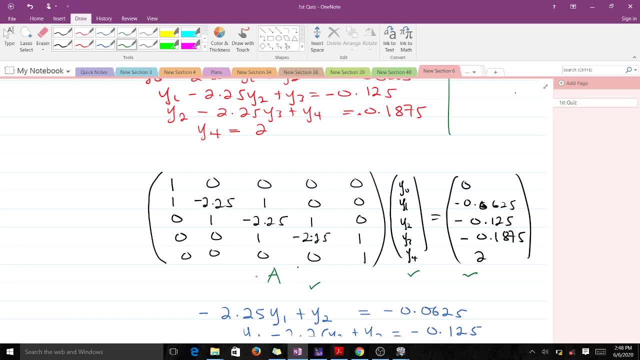 But if this would be very difficult for you to do, then you know you have values for y, naught and y4 already, So you can use that to reduce this five equations, five systems of equations, into three right? So actually, when you solve this using any method that you know you are going to get y1 to be 0, y naught to be 0, y1 to be 0. 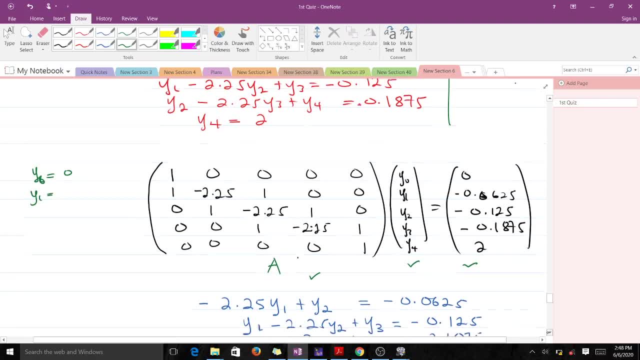 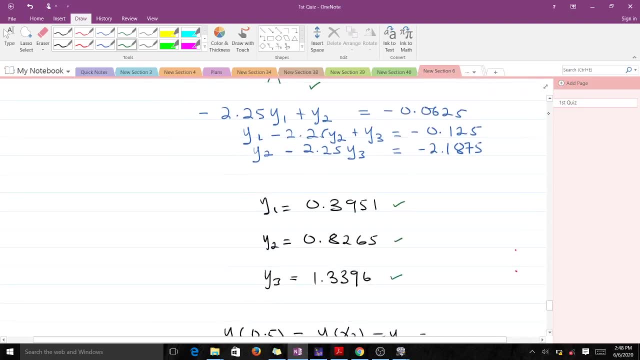 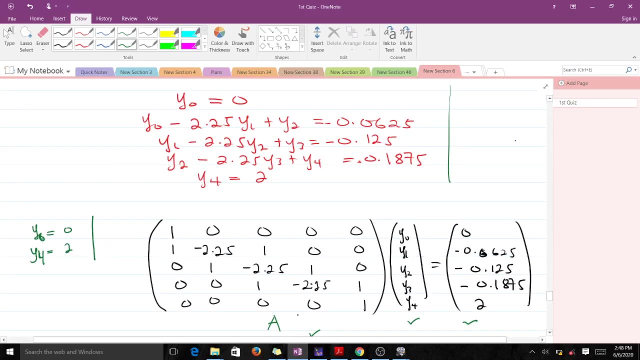 Right, So have the values here: y1 to be this, y2 to be this, y3 to be this and y4. So y4 to be 2.. Because we know y4 is equal to 2.. So since we already know the values for this, we can use that to reduce this five equations into three equations. 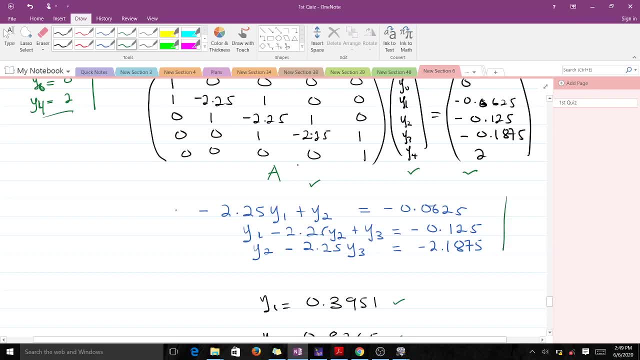 So when we do that, we are going to end up with this particular system of equations here. I hope you understand. So wherever you find y naught and y1. In equation 2. You put 0 there because it is 0. 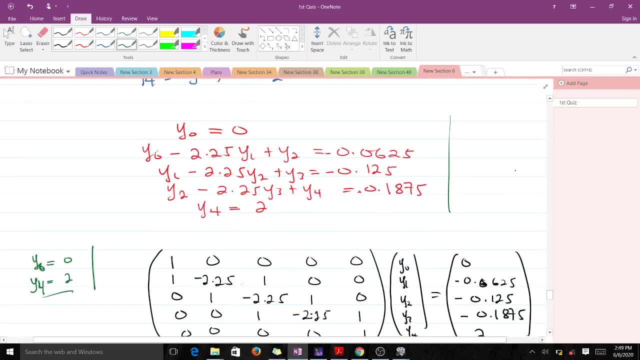 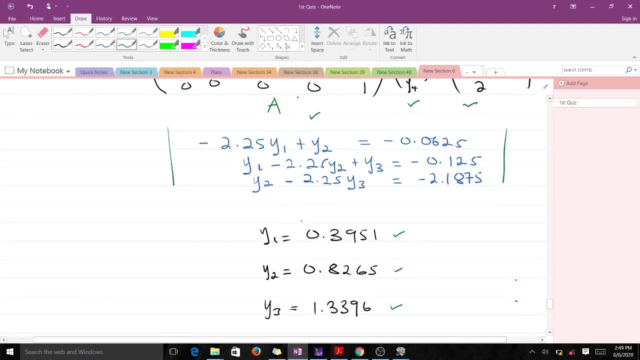 Wherever you find y naught here, you put 0 there. Wherever you find y4 here, you put 2 there. That is going to give us these three equations that we have here. So solving these three equations using any method that you know for solving systems of linear equations. 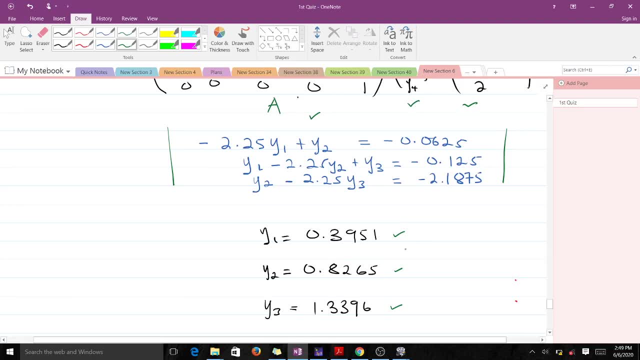 Is going to give you y1 to be 0.3951.. y2 to be 0.8265.. And y3 to be 1.3396.. Recall that we already know the values for y, naught and y4.. 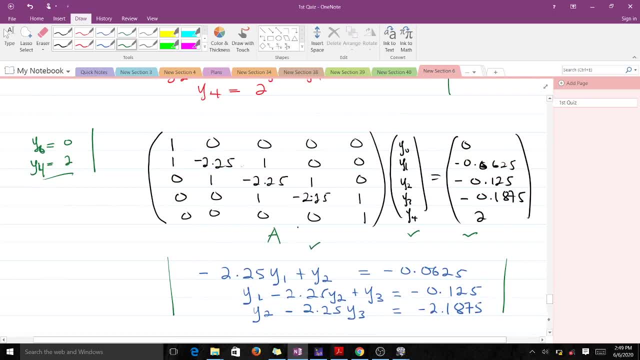 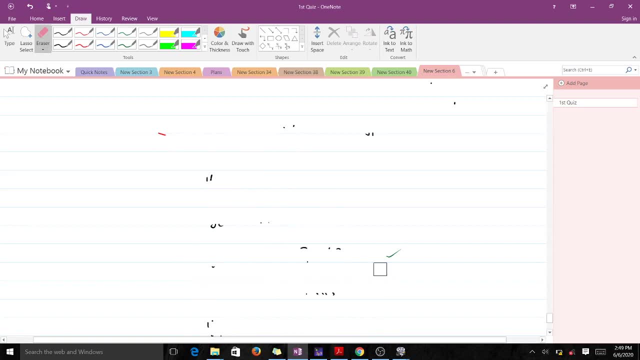 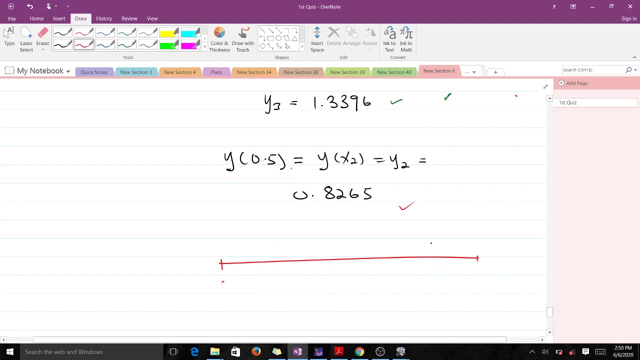 From the boundary conditions which was given to us. So let me show you something here. Remember the question said we are supposed to. So we had x between this interval 0 to 1.. And it was divided into 4.. This was 0.25.. 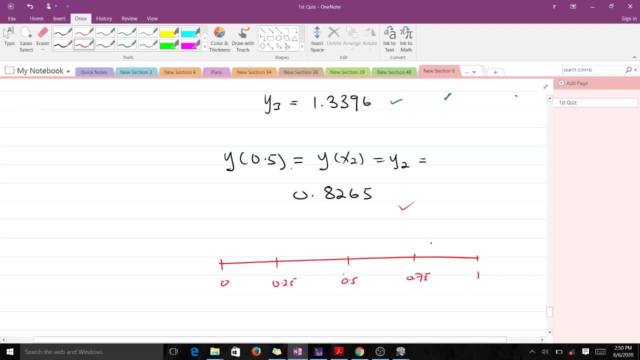 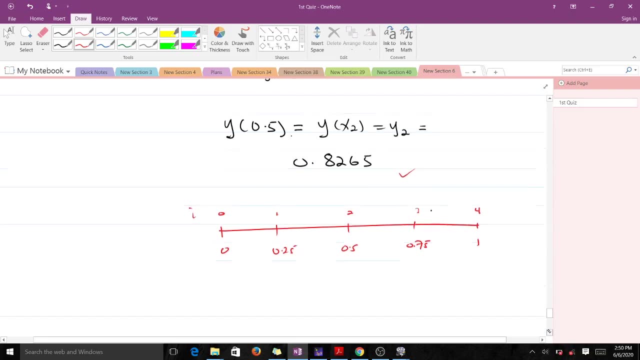 This was 0.5.. This was 0.75.. And this was i equals 0,, 1,, 2,, 3, 4.. The question said we should find the value for x at x equals 0.5..